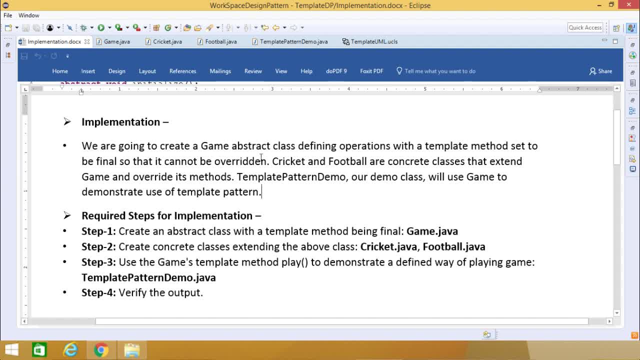 here. So here, in this project, we are going to create a game, abstract class defining operations with a template method set to be final so that it cannot be overwritten. So template method will be of the type final, so that it should not be overwritten. Cricket and football are the concrete. 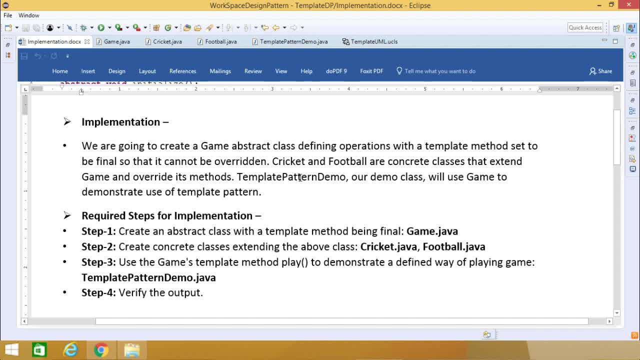 classes that extend game and override its methods. Template pattern demo. our demo class will use the game to demonstrate the use of the template pattern. So for the better understanding, let us explain line by line. Step one: create an abstract class with a template method being final, that is. 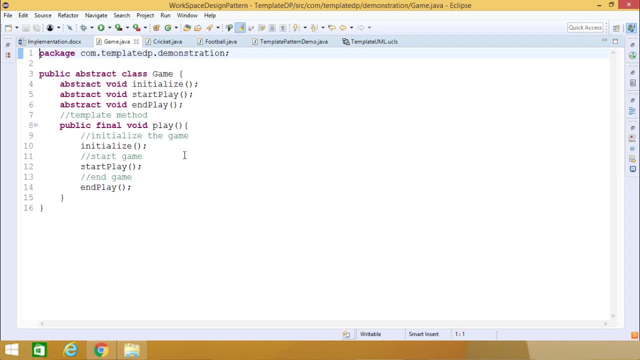 a gamejava. So here we are having this gamejava Here. this particular class game is abstract type because it is having three abstract methods. So they are: initialize, start play and end play. You can easily see their prototypes And this is the template method, which is of the type final It. 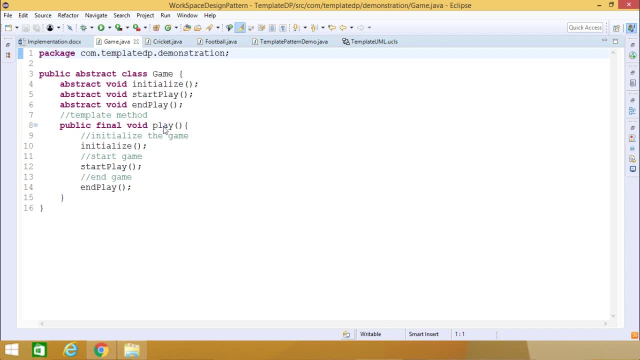 cannot be overwritten. So public, final, void play, which is having three methods called in a certain order. So this is the template method which is of the type final, It cannot be overwritten. So initialize, then start play and then end play. So in this way these three abstract methods are. 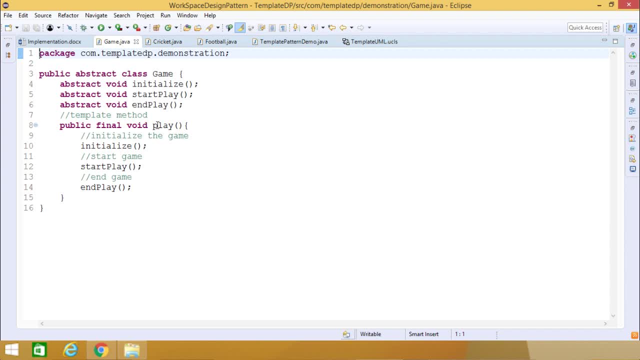 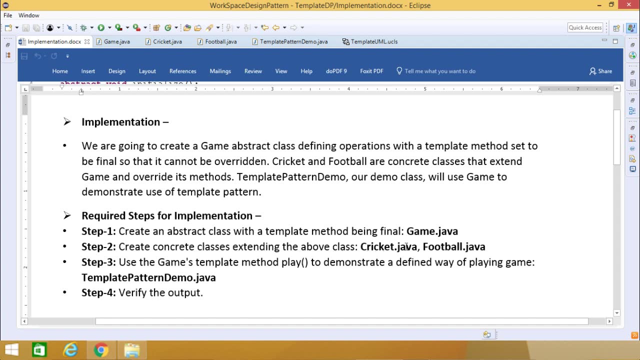 called from this public final void play. Now we are going for the step number two: create concrete classes extending the above class cricketjava and footballjava. So this abstract class gamejava will get extended here in cricketjava and footballjava So you can easily find that public. 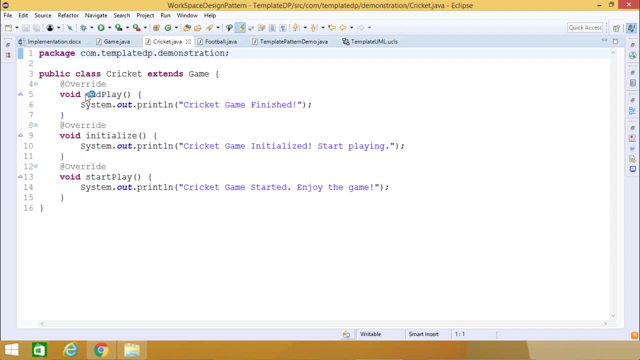 game and all those three abstract methods have got defined here. So end play. you can see the code here, Only the systemoutprintln we have written. Initialize and start play. Similarly we are going for this footballjava, and here also we have defined the respective function bodies Three: 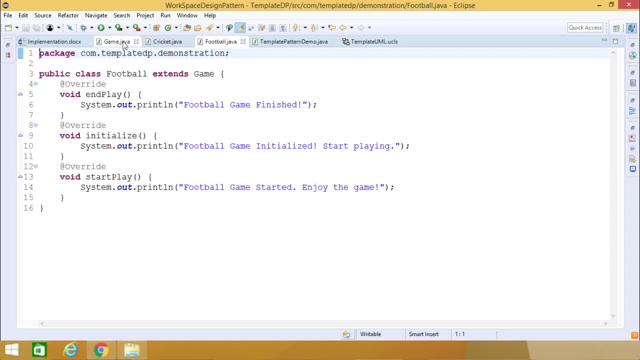 function bodies. three abstract functions were there. methods were there in our game and the bodies have got written for those abstract methods. Next we are going for this: implement implementation. So that is our step number three: Use the games template method. play to. 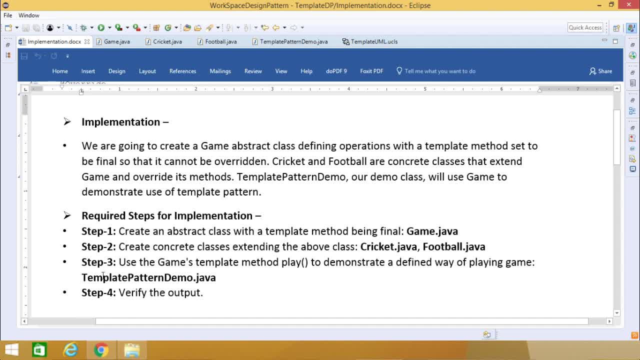 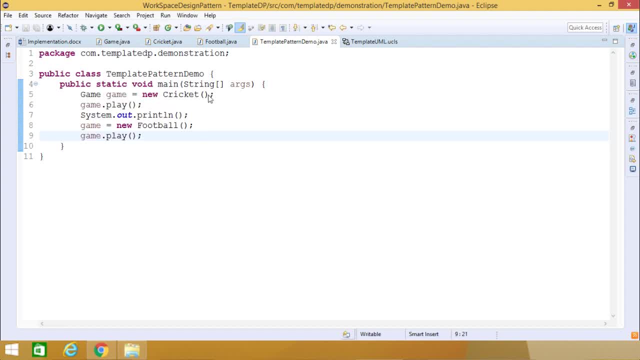 demonstrate a defined way of playing game. So go for template pattern demojava. So this is our template pattern demojava. So game game is equal to new cricket gameplay. So what will happen? Play will be calling this: initialize, start play and end play. Next we are having this: systemoutprintln. 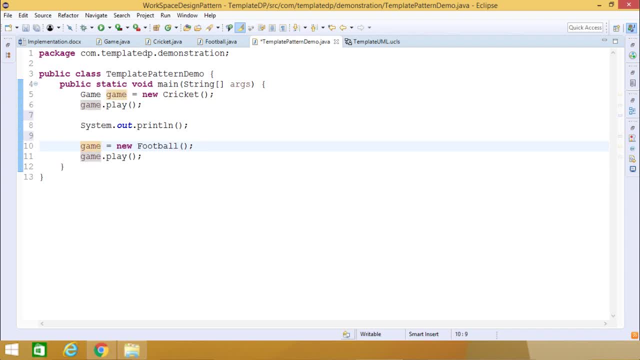 just only to bring one blank line. So now game is equal to new football and gameplay. So at first, this particular interface object is getting instantiated by this implemented abstract class object cricket- Here also abstract class object, football- and then we are going for this gameplay. So this is a template. 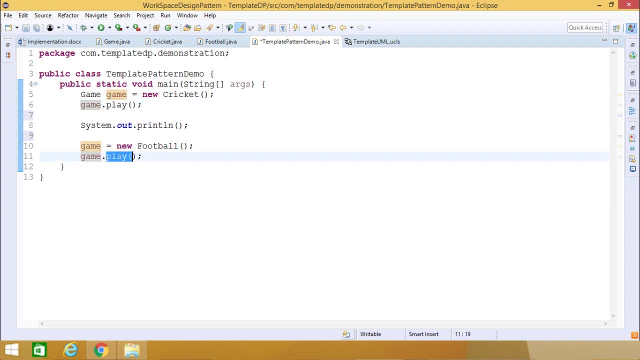 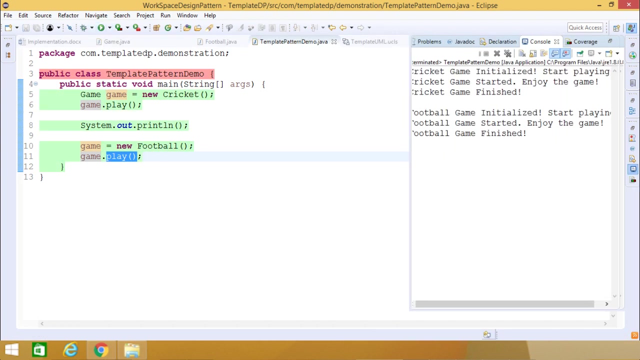 function and this particular template function must be of type final type. You can easily find that we have written the same. So public final void play. So now, if I execute the code, get the output. So here we are having this respective outputs, are there? So cricket game. 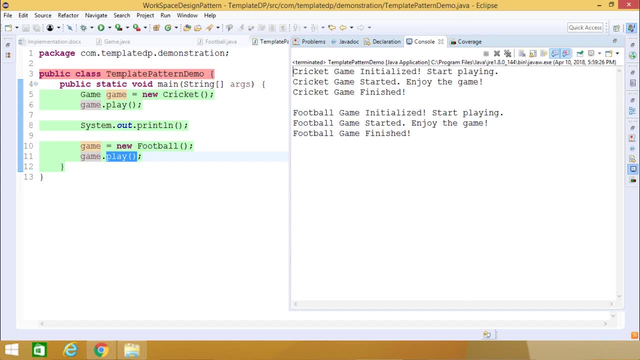 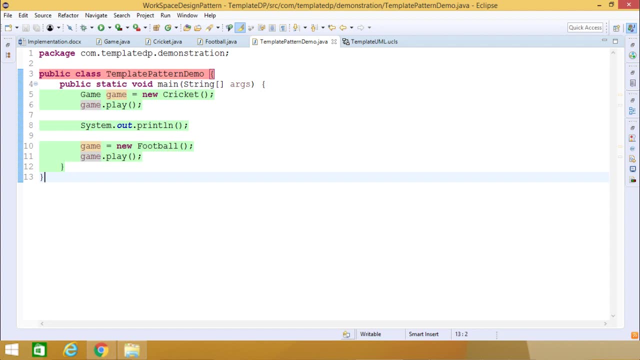 initialize, start playing Cricket game started, enjoy the game and cricket game finished, and similarly, we are having the same for the football. So in this way we are getting this respective outputs. and now let us go for this template: uml. that is a class diagram. So this is the class. 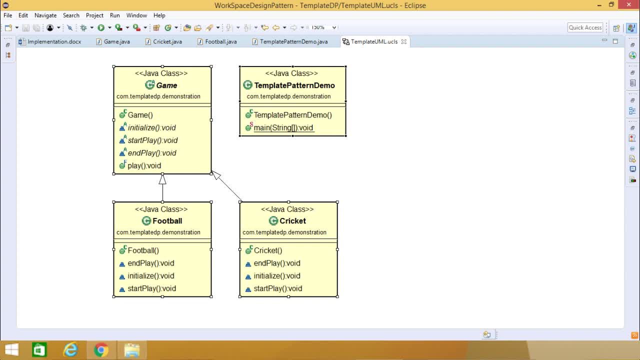 is there. We are having this final method display. These three are the abstract methods and game is constructed, So this particular abstract class. So here a denotes it is an abstract class. It has got implemented in football and cricket, two concrete classes We are having. 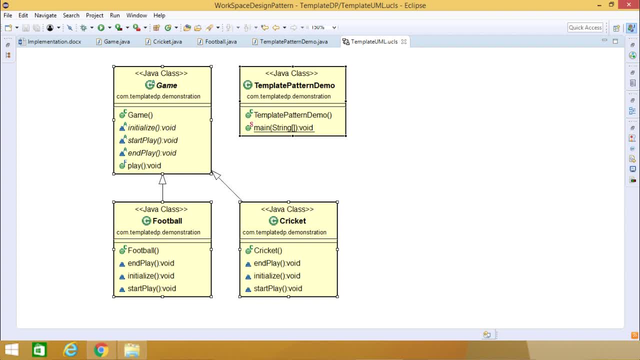 this pattern, template pattern demo and these are respective constructor and the static main function. So it is depicting that the how the classes are related. in this class diagram and in our demonstration we have, we have shown you that in using java, how this template design pattern can be implemented. Thanks for watching this video.